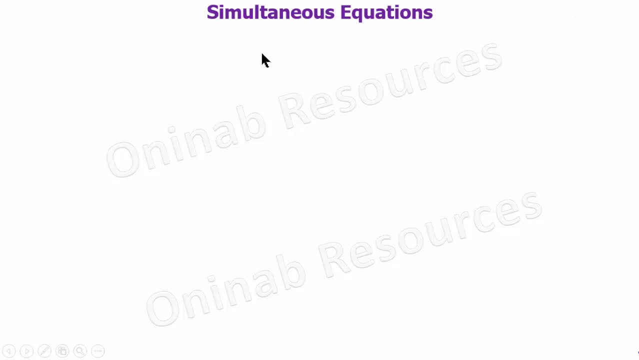 Hello out there. Welcome to this tutorial on simultaneous equations. In this video we'll be looking at graphical method. So we have our first problem, Problem 1.. Solve the pairs of equations 3x plus 4y equals 10 and 3x minus 2y equals 4 graphically. 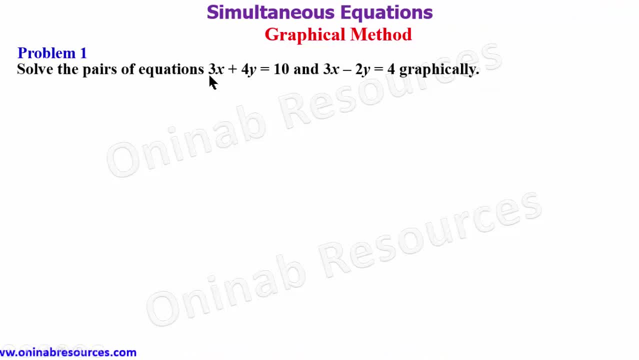 So we are going to draw the graphs of this straight line and the other straight line. Then, at the point of intersection, the coordinates will give the solution to the simultaneous equations. So we start the solution by creating the table of values for the two equations. 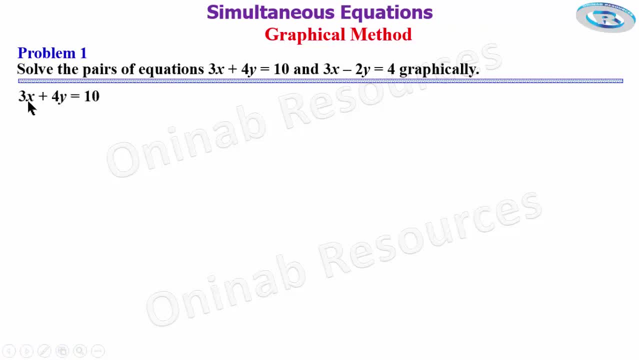 So we have the table of values, So we have the table of values. So we have the table of values. So if x is 0, we are going to have fraction here. And also, if we make y equals 0, we are going to have x to be a fraction. 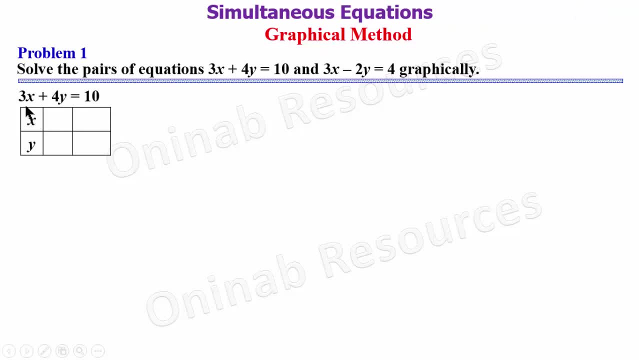 So to avoid fraction, we go for any other two points From here. this is 10 and this is 4y. If I make x to be equal to 2, I'm going to have 6 here, And on x, I'm going to have 6.. 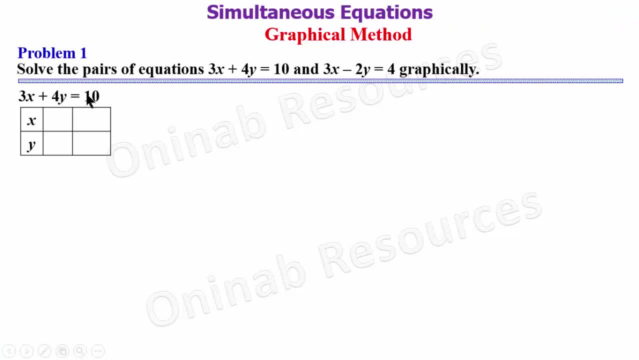 And, coming to this side, it will be 10 minus 6, which will give us 4.. From there, it is divisible by 4,, which is the coefficient of y. Therefore, if we make x equal to 2, and we say this is 6,, coming to this side, it becomes 10 minus 6.. 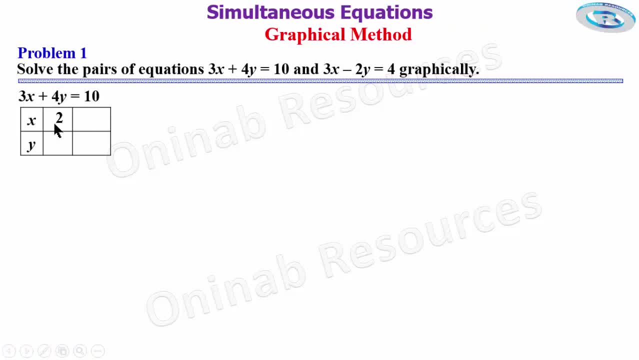 10 minus 6 is 4.. 4y will be equal to 4, where y will be equal to 1.. We have gotten the first point, Then 4y And for the second point, but we are trying to maintain small values. 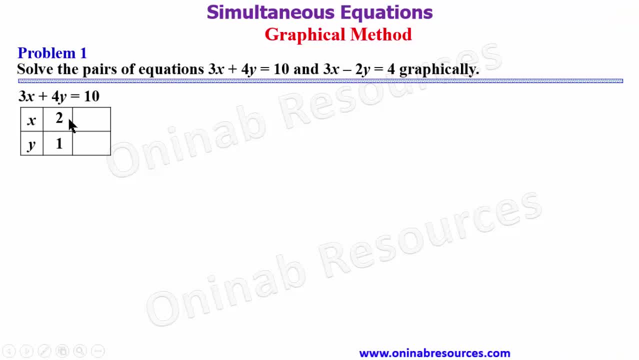 We don't want to take a very large value. that will make our range of values of x to be so large that we will not be able to contain our graph. So we pick: x is negative 2.. If we pick x is negative 2, we are going to have negative 6 here. 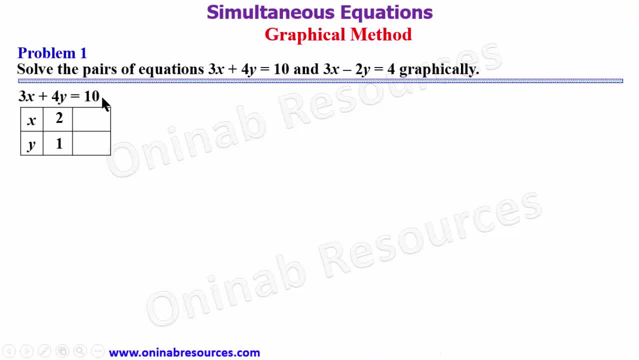 And it's bringing it to the right-hand side- becomes positive, So that we now have: 4y is equal to 16. And 16 is divisible by 4. So we make x equal to negative 2. And our y is going to be 4.. 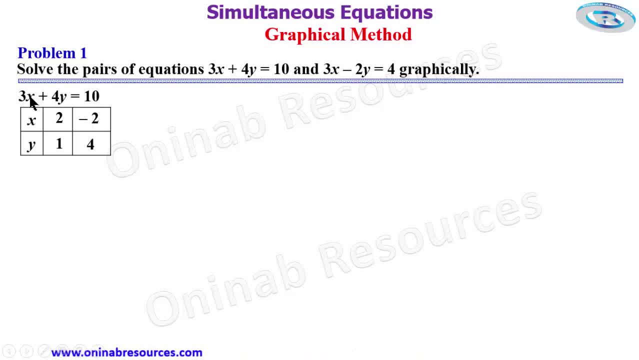 Remember, put x is negative 2, here You have negative 6.. Coming to this side, it becomes 10 plus 6, which is 16. And 16 divided by 4 gives this 4.. So we've gotten the two points to draw this line. 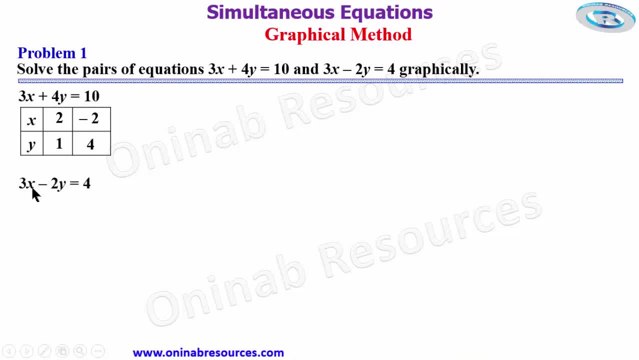 So we go for the second equation, which is: 3x minus 2y is equal to 4.. So we still come up with our table And in this case we can make x equals 0.. If you make x equals 0, this 3x is gone. 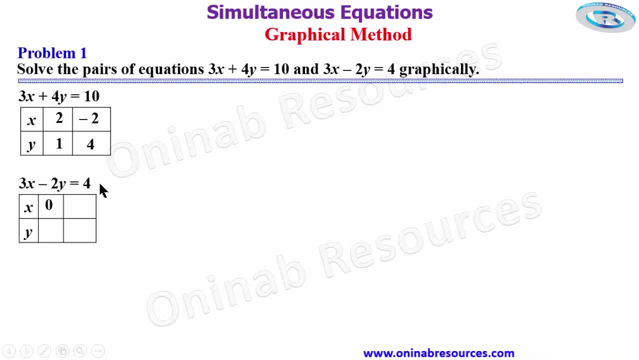 We'll be left with negative 2y. 2y is equal to 4.. Dividing both sides by negative 2, we have y to be equal to negative 2.. Now we cannot make y equals 0. We are going to have fraction. 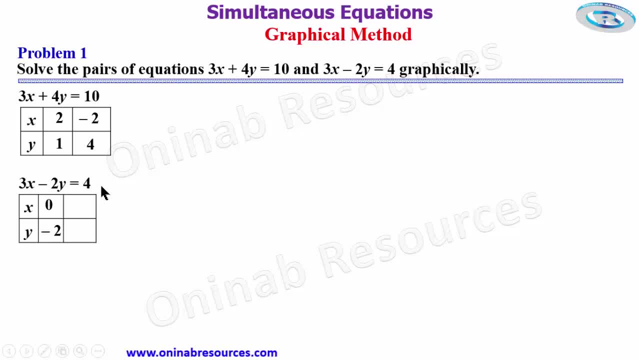 And I would find it difficult to get the fraction of the graph. So let's go for something easier. But if you can bear the pain of getting the fraction from your graph, please don't hesitate. Just go by the Intercept Form. Now we want to make x to be equal to 2 again. 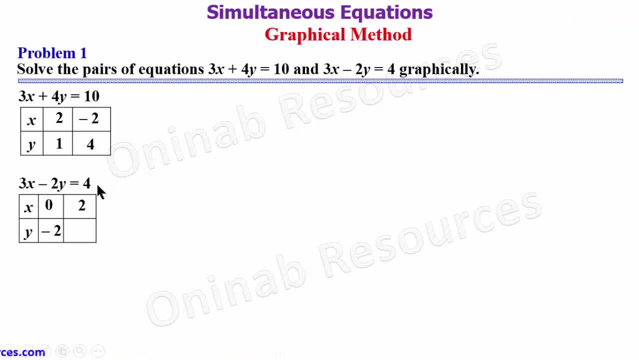 This is going to give us 6.. 6 goes to the other side. It becomes 4 minus 6, which is negative 2.. So we now have negative 2y is equal to negative 2. And at that point y will be equal to 1.. 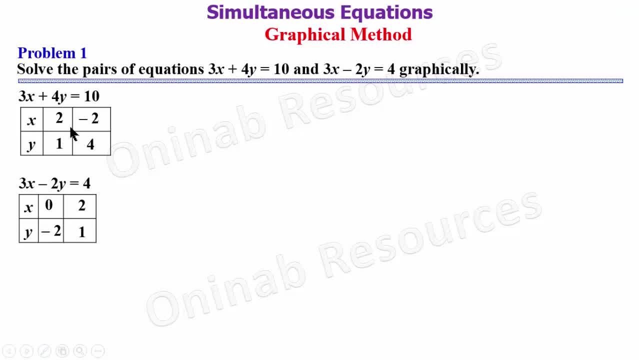 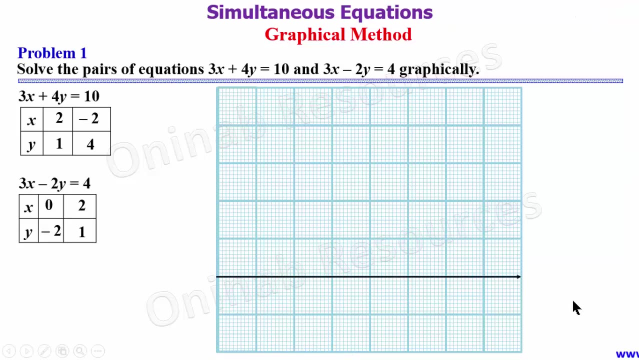 We can then go ahead to plot this point to get our straight line here. Okay, we also plot the two points here to get our straight line. so we have our graph here. so this is our graph. we have our x axis and our y axis. you have to be very careful. 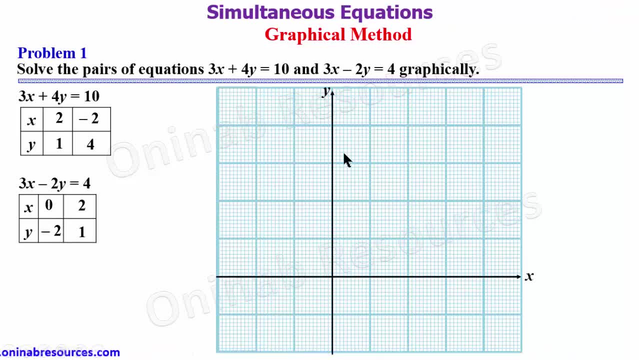 where to place x axis and y axis. we have treated graphs of linear equations, so you check our youtube channel to get them and this is the origin. to the right we have one, two, three, four, and to the left of x axis we have negative one, negative two and to the upper part of y we have a positive one. 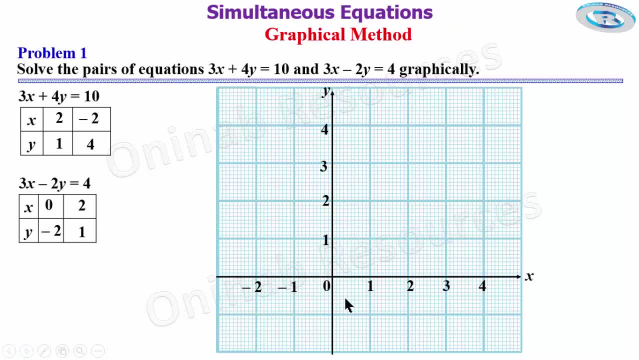 two, three, four. and to the negative side, we have negative one, negative two. then we start with the first point here, which is two. one meaning when x is two, y is one, so the line x is equal to two. is this: this is: the line x is equal to two, so the line y is equal to one. is this: you see, they meet here, so we mark the point out. 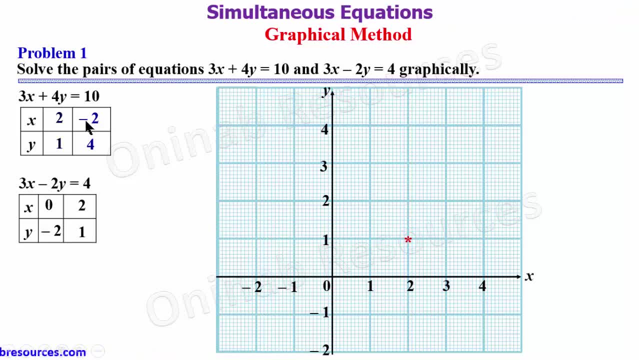 then we are done with that point. we go to the second point, that is negative two and four. the line x is negative two is this, and the point is here, since y is four here. so they meet here. we mark the point also. we then place our ruler from. 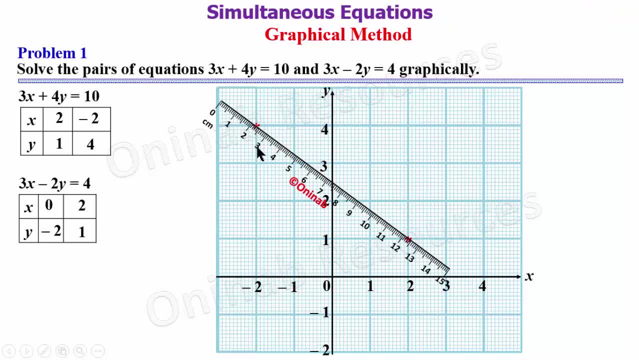 touching the first and the second point. then we draw our line, so we have the line: 3x plus 4y is equal to 10. this is the line. so we go to the second equation, which is also a straight line. the first point is 0 and negative 2. x is equal to 0, is y axis, this is: x is equal to 0. 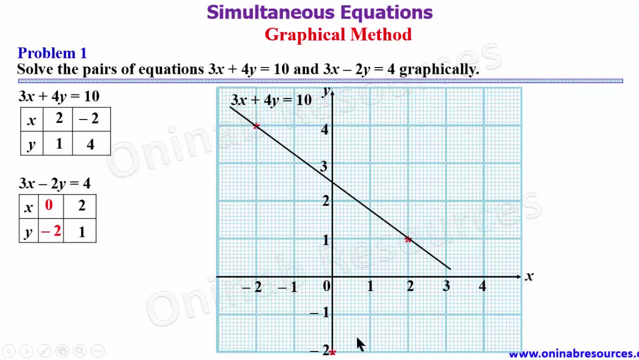 y is negative. 2 is this point, so i mark the point out. then we'll go to the next point, that's: uh, two and one. when x is two, y is one is a repeated point as we have it here. so this is the point here. so we just place our ruler again. 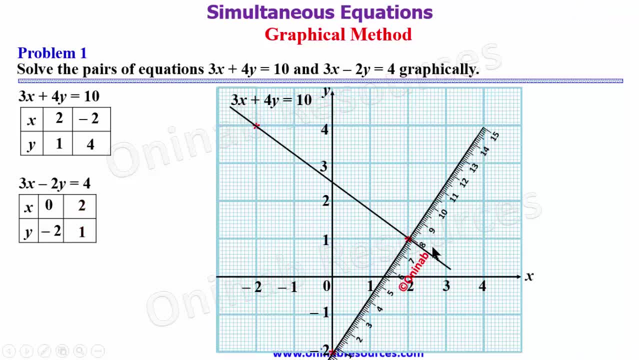 and then join the two points. make sure you extend it as long as possible. so we are done. drawing the second line, which is 3x minus 2y, is equal to 4.. so the solution here now is the point of intersection of the two lines. we get their. 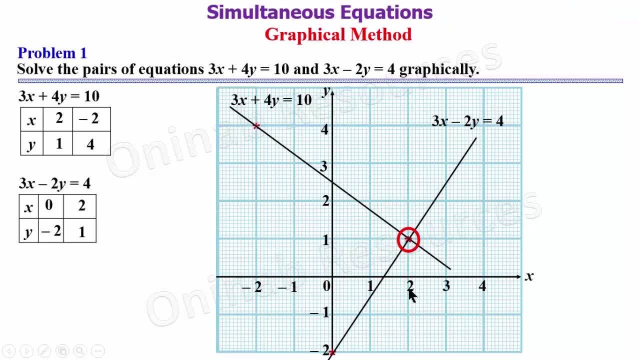 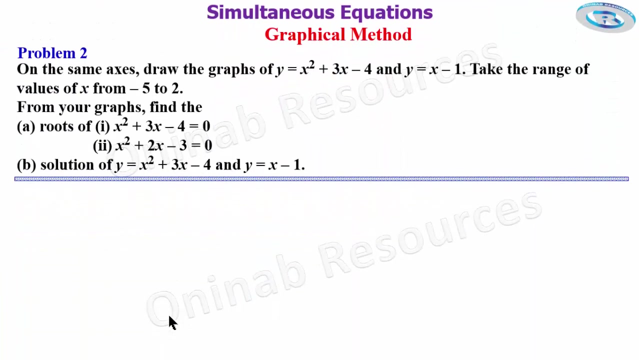 coordinates, which means that point, the value of x and the value of y, so that the solution is two. this is two. the point is two to the x-axis and one to the y-axis. so that's the end of solution to problem one. we then go to problem two. 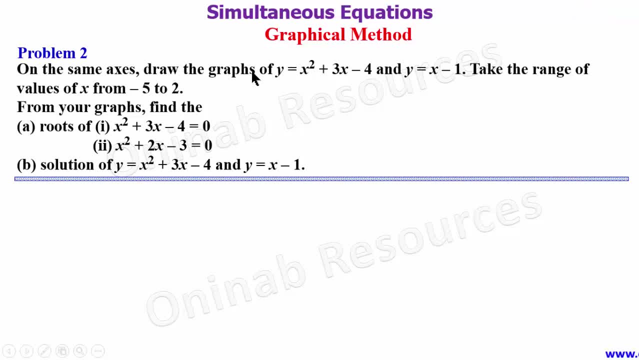 for problem two, on the same axis, draw the graphs of y equal to x squared plus 3x minus 4, and y equals x minus 1.. take the range of values of x from negative 5 to 2 from your graphs. find the roots of 1. x squared plus 3x minus 4 equals. 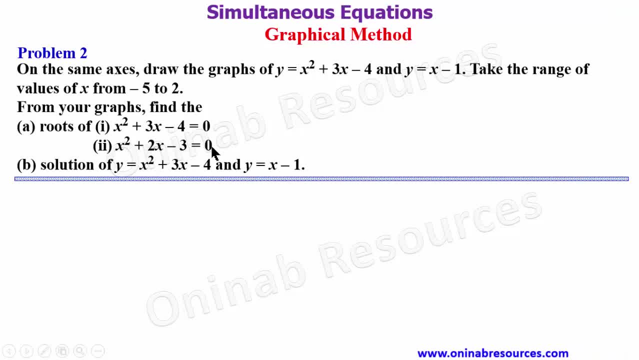 zero two. x squared plus two, x minus three equals zero b. we have to find the solution: of y equal to x squared plus three, x minus four and y equals x minus one. we have two equations here. this one is a curve, a quadratic curve. why? this is a straight line, so this is a situation of simultaneous. 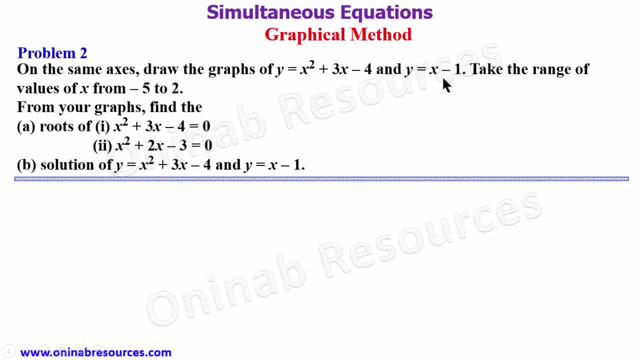 equations, one linear. this is linear and the second one is non-linear. so we've treated the analytical solution in our previous videos. check the description section of this video on our youtube channel to get the previous videos on simultaneous equations. so we start with the solution. so we are going to create table of values. 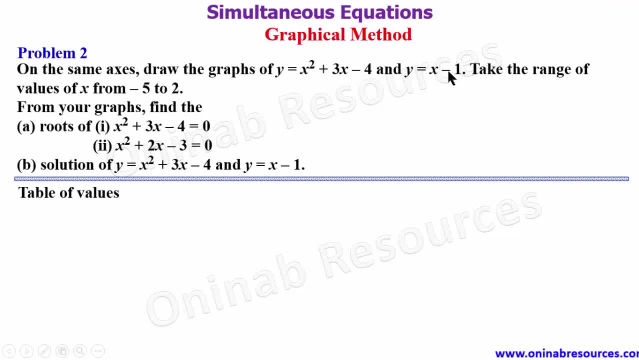 so for the two equations, the curve and the straight line. so we start with the curve. we are going to have an expanded table. for the table of values. i love using this method, but you can use your calculator to be faster. but for the purpose of this video i want us. 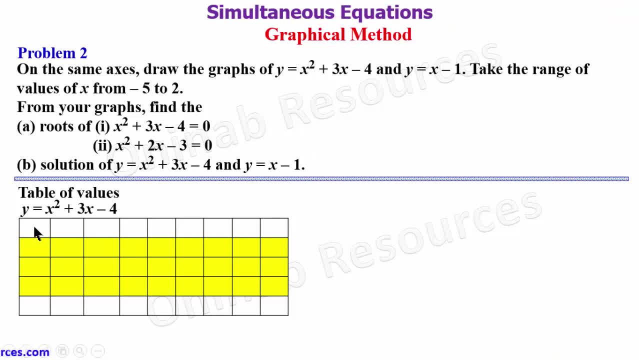 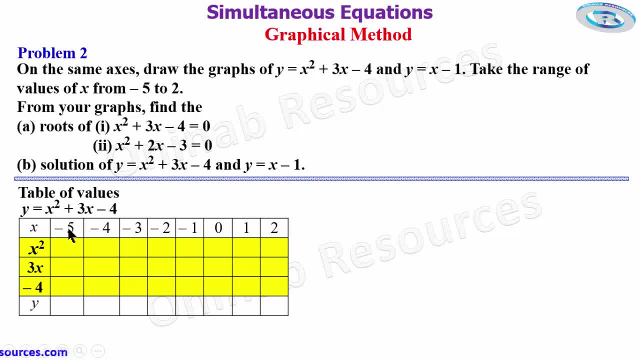 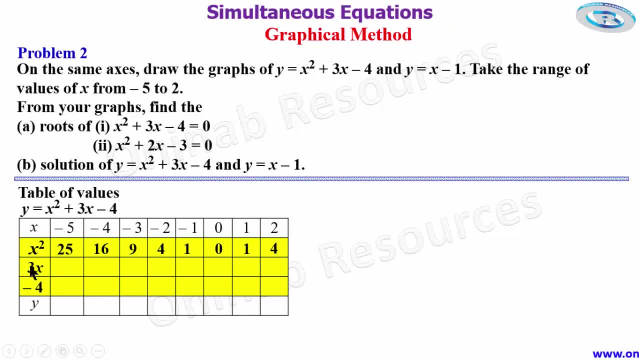 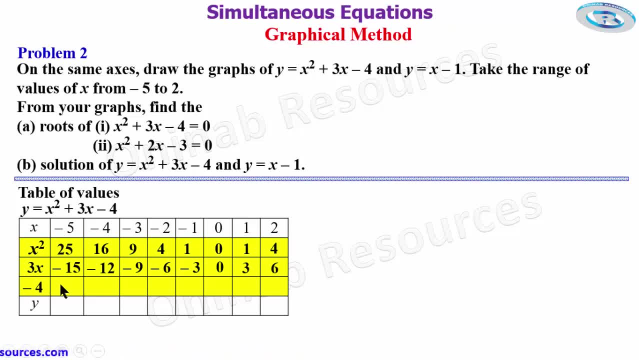 and three times two gives six. and for this constant term, we are going to repeat all of them for each of the cells. okay, so we are done. then we now add up the calculated values. that's 25 plus negative, 15 minus 4. that will give us 6, 16 minus 12. then minus 4 gives 0. 9 minus 9, 10 minus 4 gives negative 4. 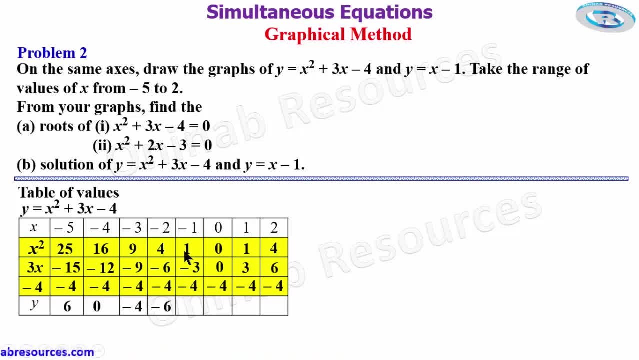 4 minus 6 minus 4 gives negative 6. 1 minus 3 minus 4 gives negative 6. 0 plus 0 minus 4 gives negative 4. 1 plus 3 minus 4 gives 0. and finally, 4 plus 6 minus 4 gives 6. so we are going to use the first. 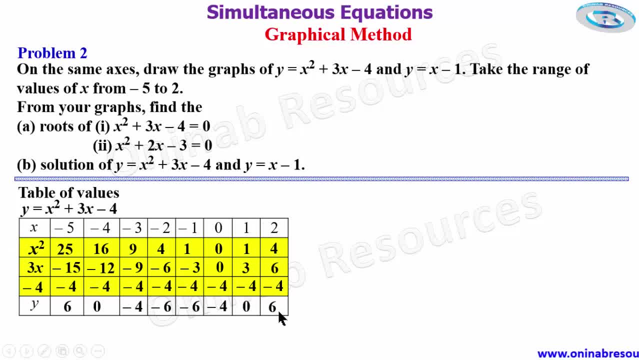 row and the last rule to draw our graph, that is the rule for the values of x and the corresponding rule for the value of y. so that's that for the table of values for the curve. then we go for the straight line. we still need two points, as we did in. 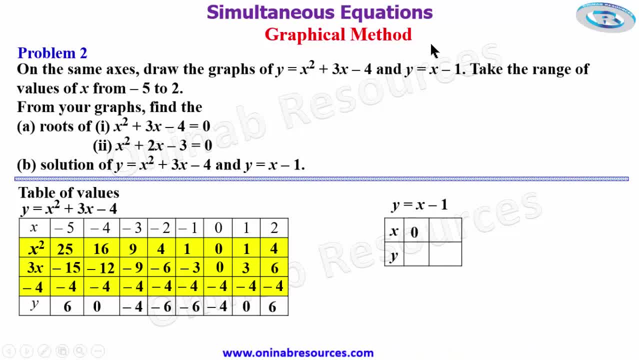 the first one. um, when x is zero, when x is zero- see, this is gone. so y is negative one. now also when x, or we say when y is zero, here, when y is zero, we have zero is equal to x minus one. we can bring negative one to this side. it becomes x equal to one. so we have our value of x to be. 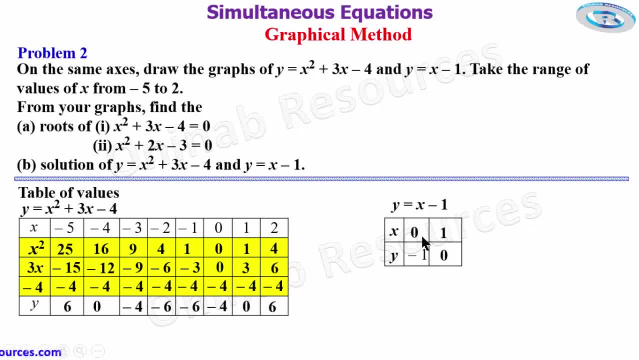 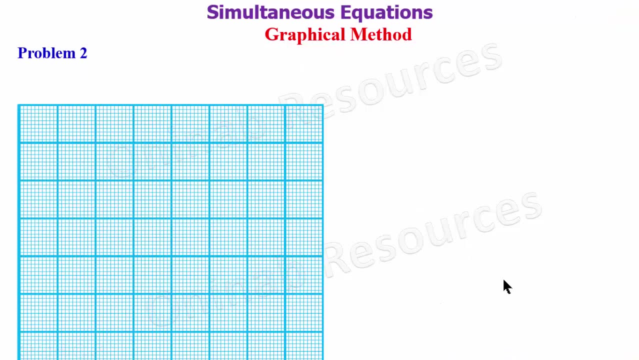 equal to one. so these are the two tables we are going to use to get our graphs ready for other questions. so we go to for our graph. so we have our graph here. remember, we have the first table, that is for the curve here, based on the values of x and y, we study the graph and get our x axis, then our y axis, if you. 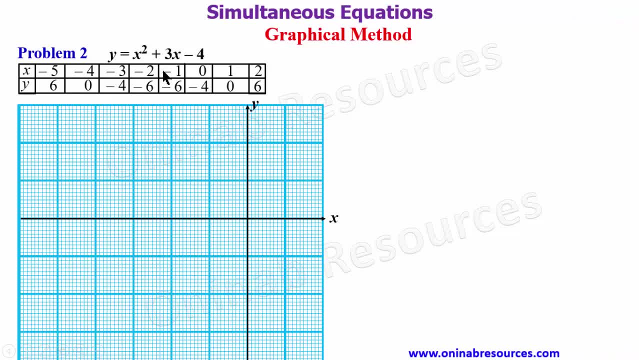 look at it now. i have more of the negative values of x, so i left more grids with the negative x axis and less here. the same thing. here we have- uh, almost equal- negative six and positive six, so we are going to have the origin. this is one and two. here is negative, one negative, two negative. 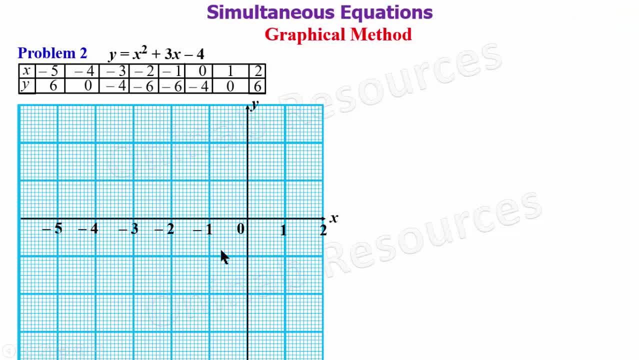 three negative, four negative, five. then to the upper part, that is positive y axis. this is two, four and six. this is negative. two negative, four, negative, six. um, i start with the first point. when x is negative, five, y is six. when x is negative, five, y is positive, we go up. this is the point, it is marked out. when x is negative, four, y is zero. this. 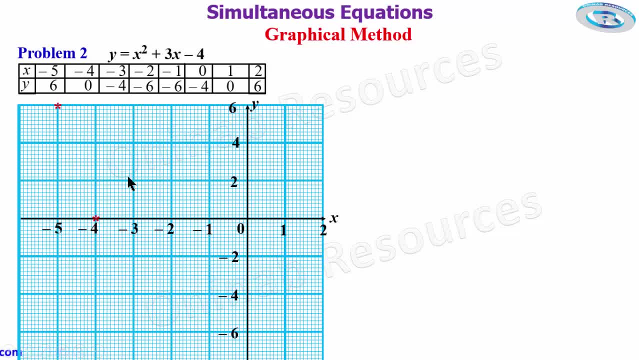 is the point here. when x is negative three, y is negative four. we go down until we get to the line y is negative four, which is this point. it is marked out when x is negative two by going down to y negative six. y is negative six is here, and when x is negative one, y is negative six is also here again when x is zero. 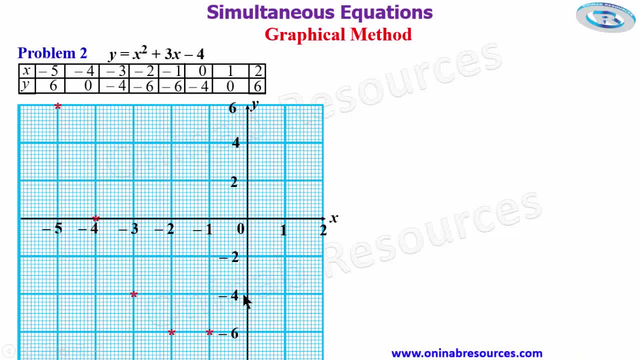 that's y axis. y is negative four there. so we have the point here. and when x is one, y is zero. this is the point. finally, when x is two, y is six. when x is two, you go up to the line: y is six. this is the. 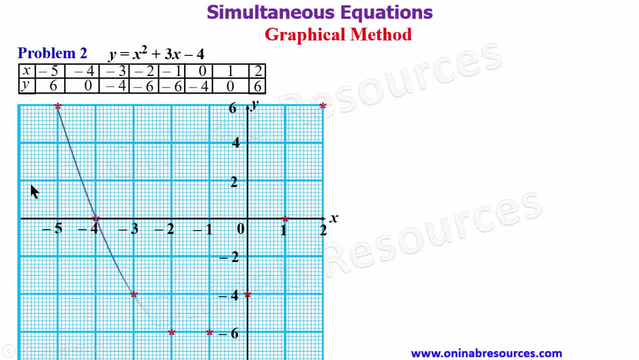 point here. then we join the points to get our curve. that is it. so that is the curve: y equal to x squared plus three, x minus four. then we go for the second table of values for the linear graph: negative one when x is zero, is y axis negative one. okay, this is two centimeter to represent two. 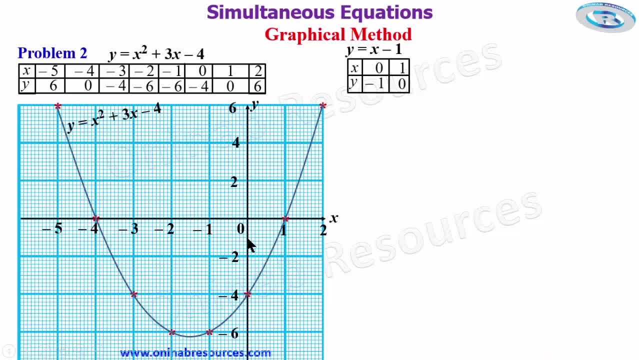 units, so halfway between them. so this is the point here. it is marked out. and again, when x is one, y is zero, y zero is x axis. so this is the point here also. we then place our ruler and join the two points, extend the line so that it covers the curve at both ends. so that is that. 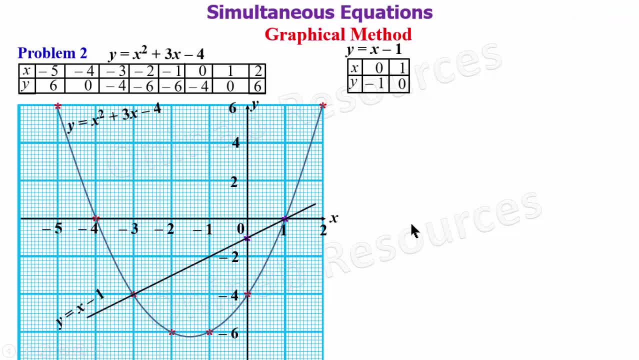 and this is y- is equal to x minus one. so we then go ahead to solve the problems that follow. so from the graphs, find the a roots: of x squared plus three, x minus four equals zero, and two x squared plus two- x minus three equals zero. so we start with a one. 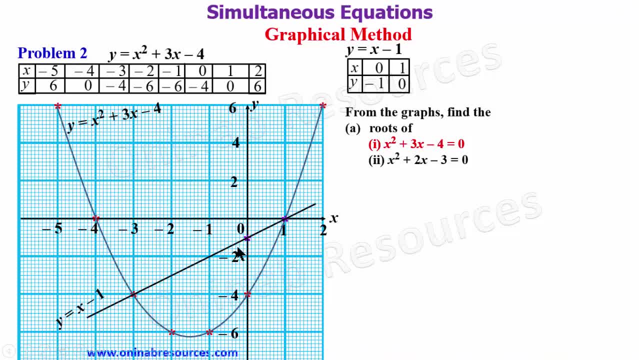 um with this. this is the curve. when we now write equals zero, we are looking at where the curve cuts the x axis, the value of x at those points. so we have the first point here and this is the second point, where the curve cuts the x axis, which represent: 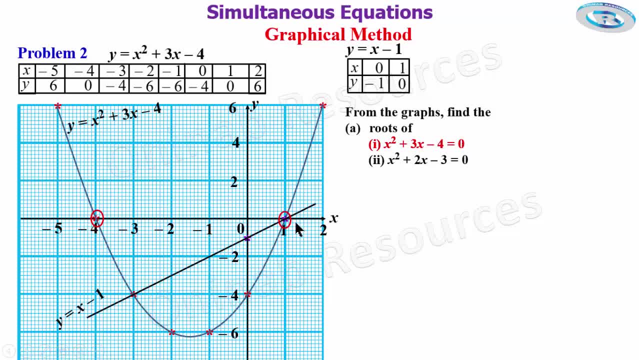 y equal to zero. so the values there now are: x is equal to 1 and x is equal to negative 4.. and that is that. so we go to a 2.. for a2 we have x squared plus two. x minus 2 equals zero. and we go to the third point here and we start with x as its. 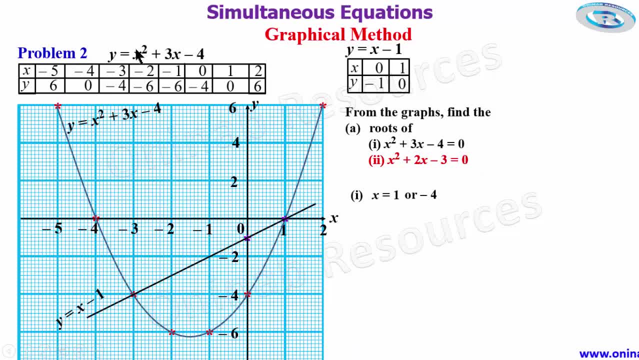 This is an equation formed from equating the equation of the curve and the equation of the line, Because if you equate x squared plus 3x minus 4 to x minus 1, simplify- you are going to have x squared plus 2x minus 3 equals 0.. 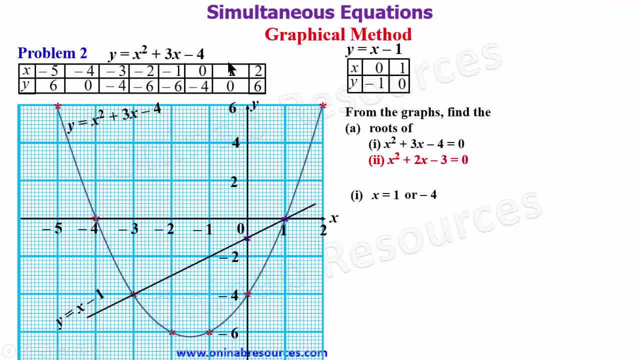 So the roots of this particular equation, formed from the two equations, are the points where the curve and the line meet. So you can see that this is the point. this is the point. So we are interested in only the values of x at each of the points.